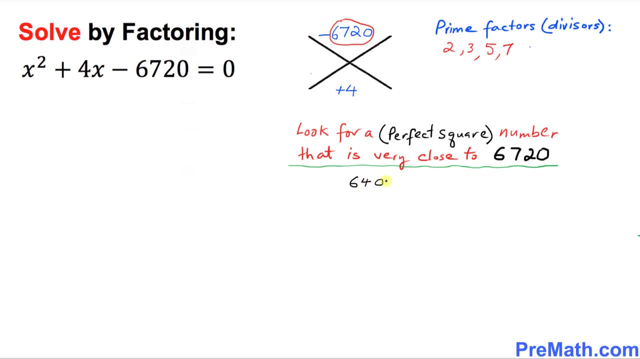 2720 is 6400.. That could be easily factored out to 80 times 80. That means our possible factors of 6720 are going to be real, really close to 80 and 80. And thus our possible factors turn out to. 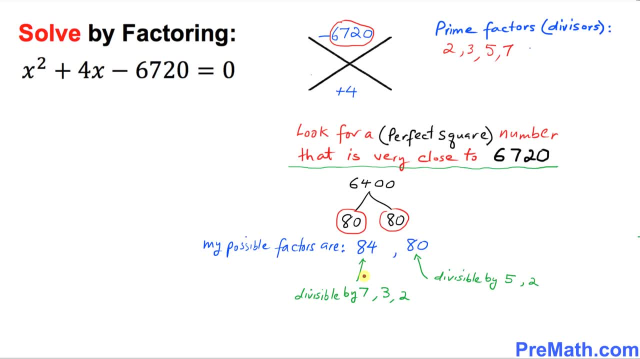 be 84 and 80.. And you can see that these both numbers are divisible by our prime factors. as you can see that one, 84, is divisible by not only 7, by 3 and 2.. And 80 is divisible by 5 and 2.. 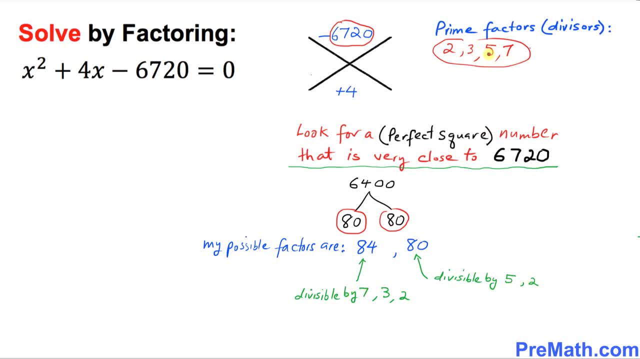 Make sure that they must be divisible by all these factors. So thus we know that our possible factors turned out to be 80 and 84.. Isn't it? And we can see the difference is positive. The only thing is we need to fix the sign So this become positive 84 and negative 80. Thus our two factors of this. 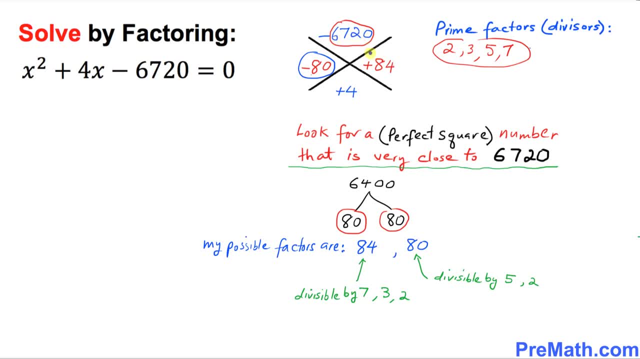 67, negative 6720 turns out to be a negative 80 and positive 84.. So let's go ahead And let's focus on this side right now. So our possible factor is going to be like this one: I want you to put down two parentheses equal to 0.. So first I want you to put down x and x And in. 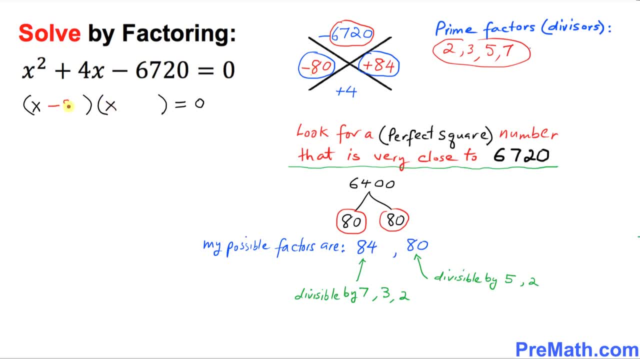 the next step. we are going to put down negative 80 in the first parentheses and plus 84 in the second. So since these two factors equal to 0, we can easily separate them. I can write x minus 80 equal to 0 and x plus 84 equal to 0. That means x turns out to be one of the solution. is x equal to? 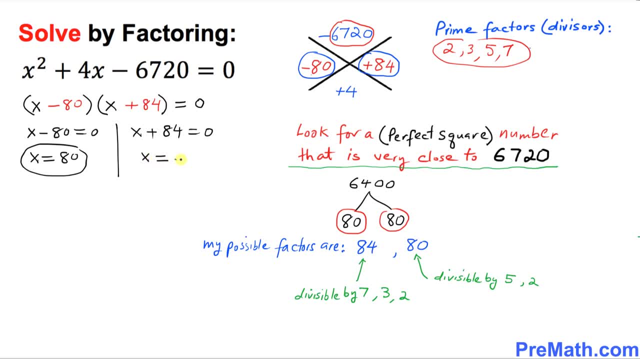 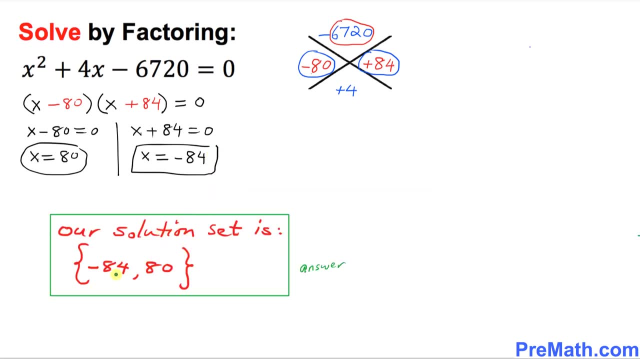 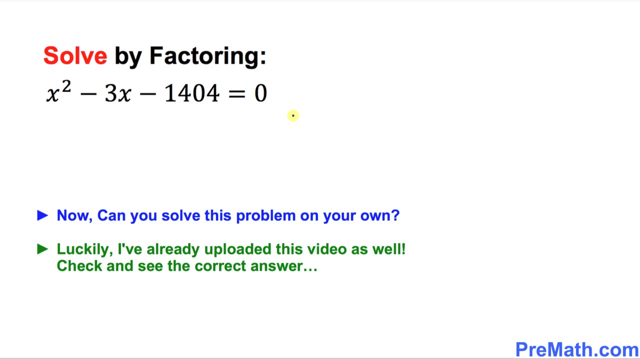 positive 80 and here x equal to negative 84. That is another solution. So thus our solution set turns out to be a negative 84 comma 80. And here is your assignment. Can you do this one on your own? You can take your time. You can pause the video. Luckily I have.